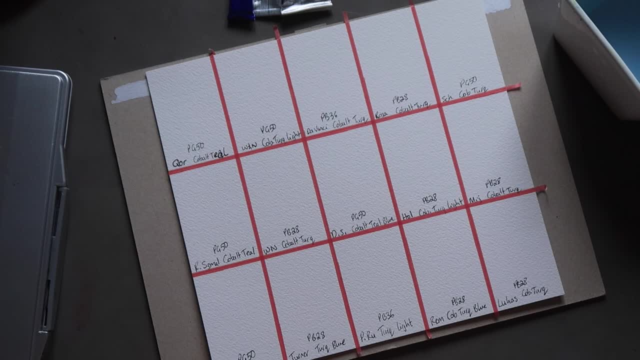 series. Um, I might have them already lined up, or if I don't and I have enough um variations of that shade to do a comparison, then I will go ahead and add it to the series. Otherwise, um, yeah, we have 15 colours to look at today, so quite a large selection. This is one of my favourite colours. 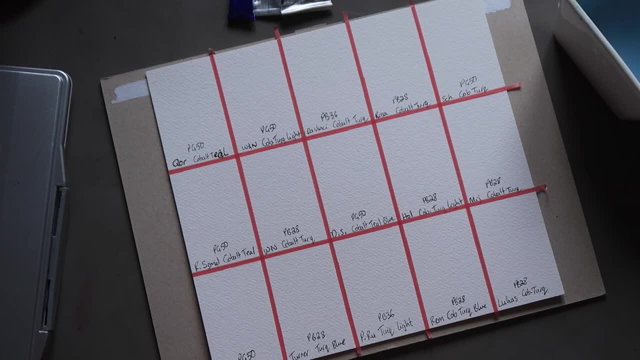 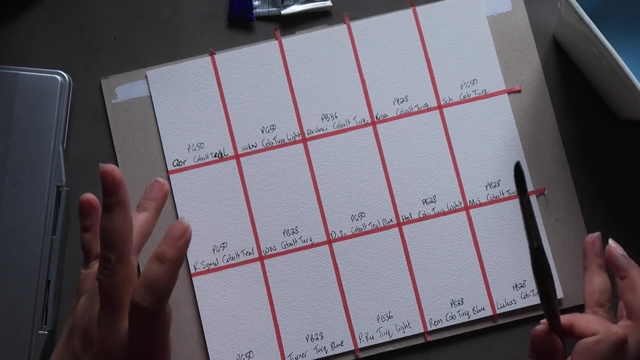 I have quite a few variations of it and yeah, and at the end, once we've done everything, I will, um, you know, once everything's dried, we'll take a look through and see which ones. well, I'll tell you which ones are my favourite. I'm using 100% cotton, arches, watercolor paper, 300gsm, cold press and 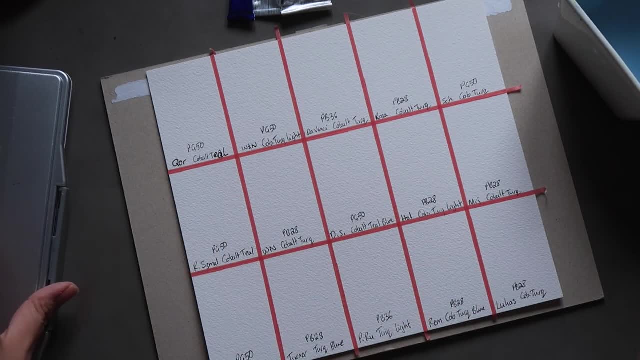 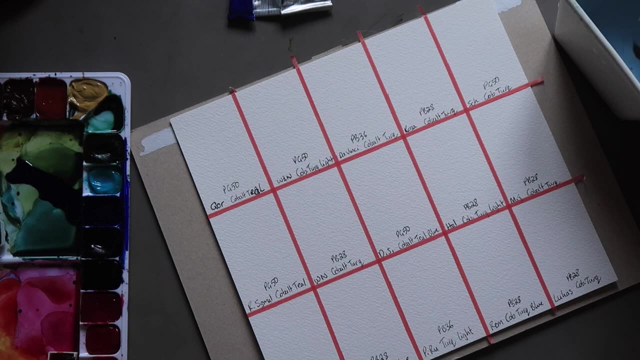 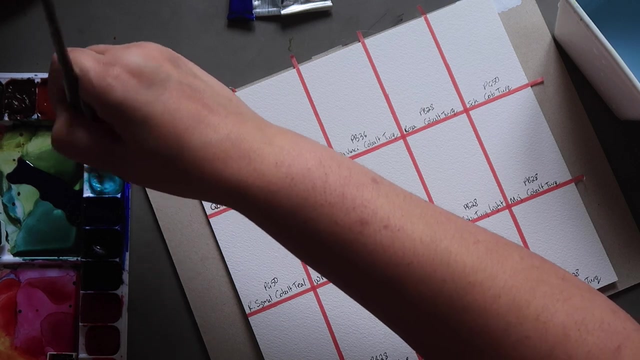 my da vinci colonea size 8 round brush for swatching today. Okay, so we're going to start first with core cobalt teal. so the core cobalt teal is PG 50. it's a really lovely one. this is a very, this is a granulating. 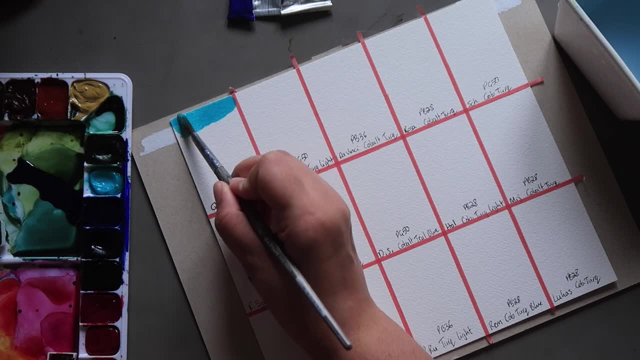 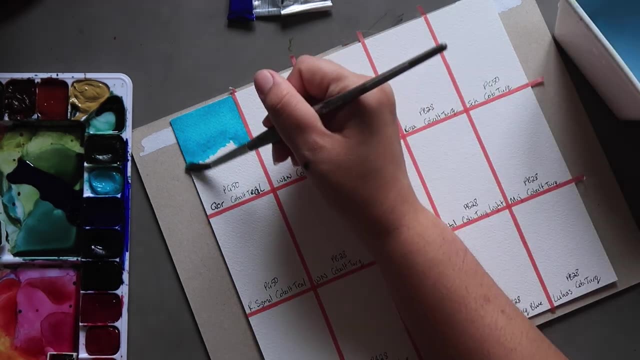 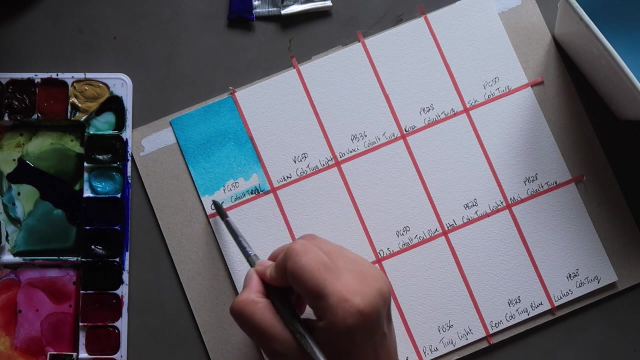 color as well, so we also be able to take a look at the variation on the granulation and see which ones granulate more compared to others, because you know, some people might want a less granulating sort of cobalt teal color and some might want to find which one is the most granulating. so 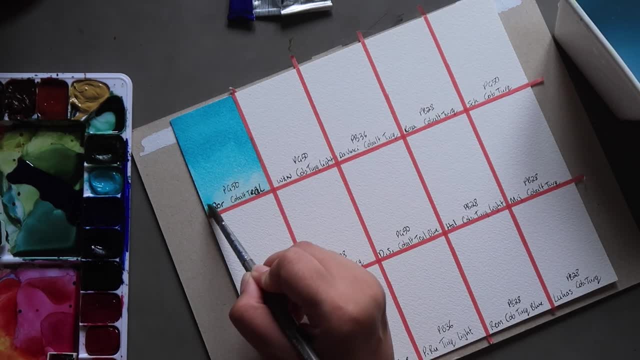 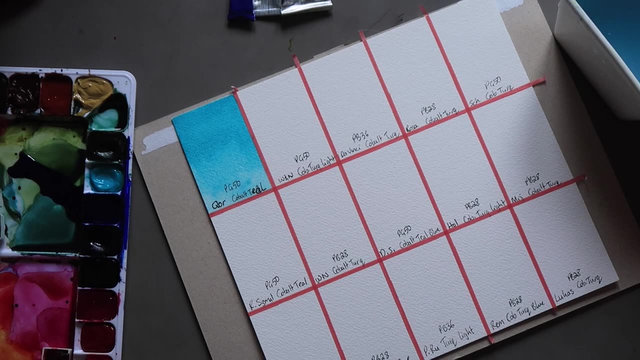 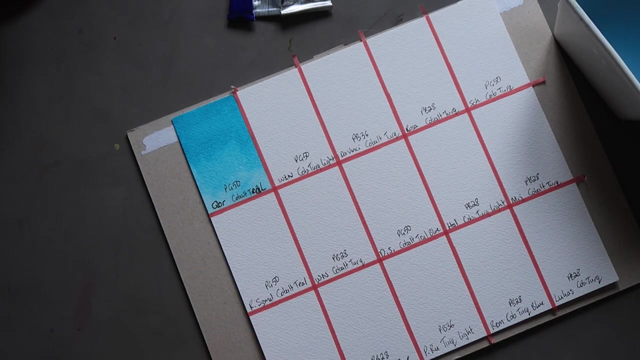 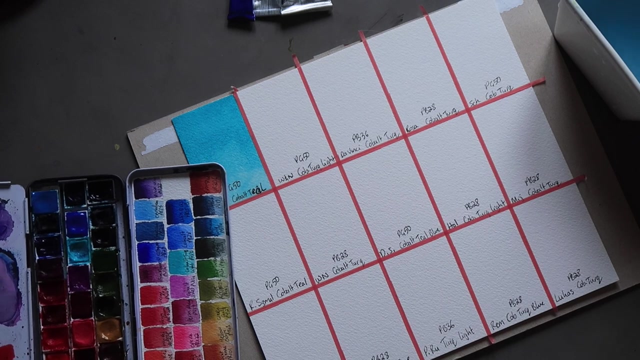 hopefully we'll be able to figure that out today. that's a really nice, quite a green leaning version. again. some of these will be more green leaning, some will be more blue leaning. okay, next up we have Winsor & Newton's cobalt turquoise light over here. 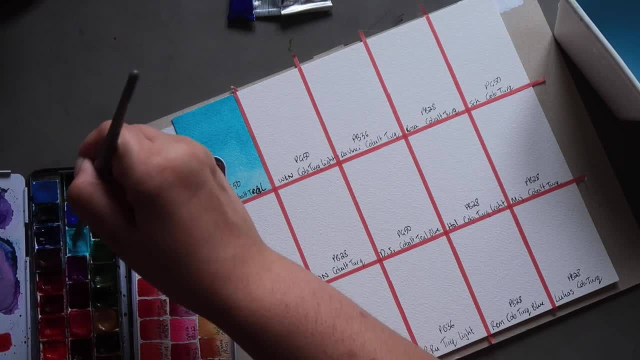 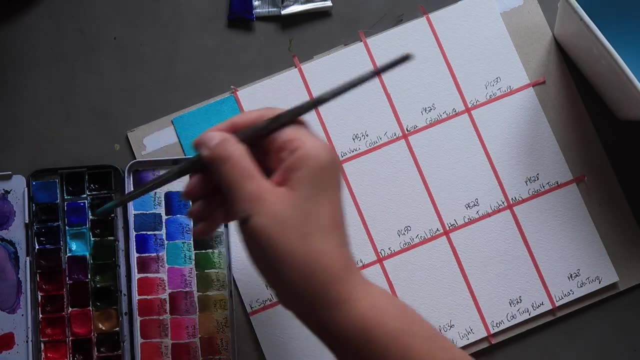 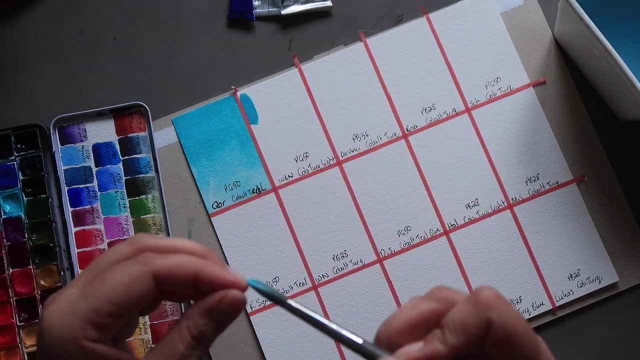 so they call this cobalt turquoise light, and they also have a cobalt turquoise which is a slightly darker, more muted greenish shade. this one is PG 50. sorry, a lid in the wet swatch there, so this one's also PG 50, same as the core. 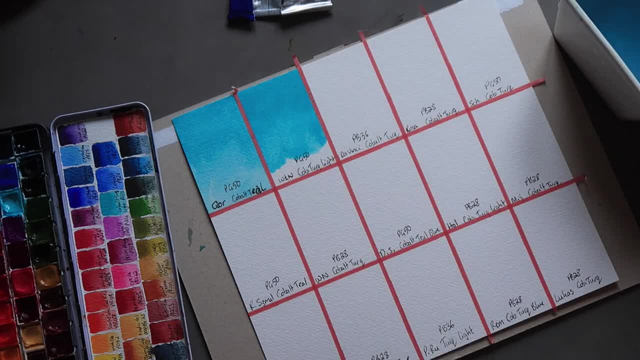 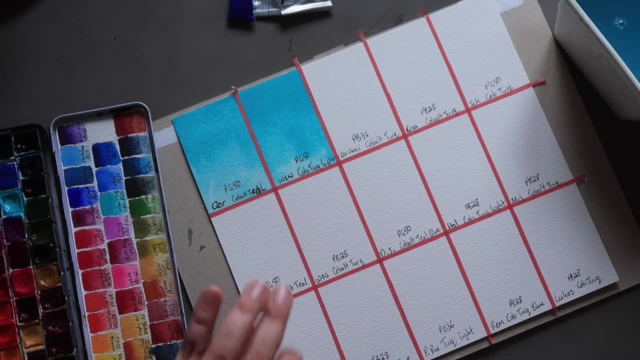 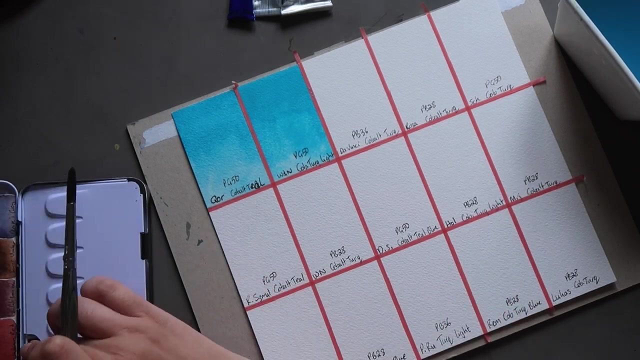 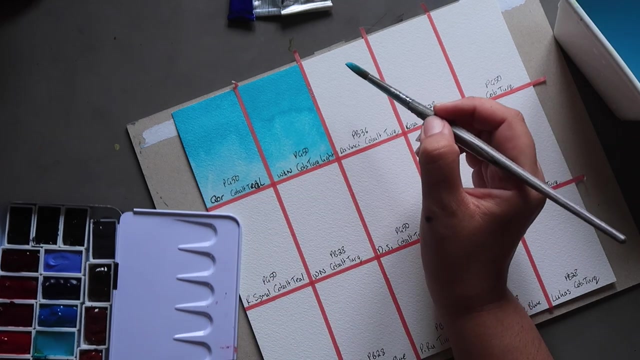 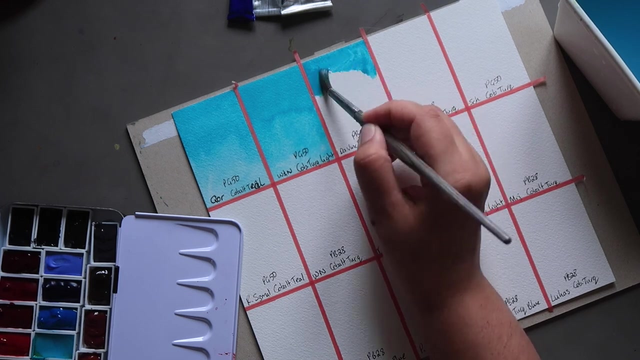 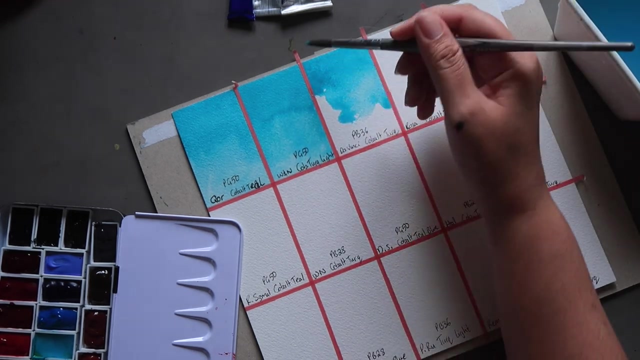 right off the bat, I'd say, this one is ever so slightly more saturated, slightly darker. then next up, we have da Vinci's cobalt turquoise. now da Vinci's one is PB 36, so PB 36 is more commonly used in um used to create cobalt. uh, sorry, cerulean blue chromium, um is. typically it is a cobalt pigment, but it's. 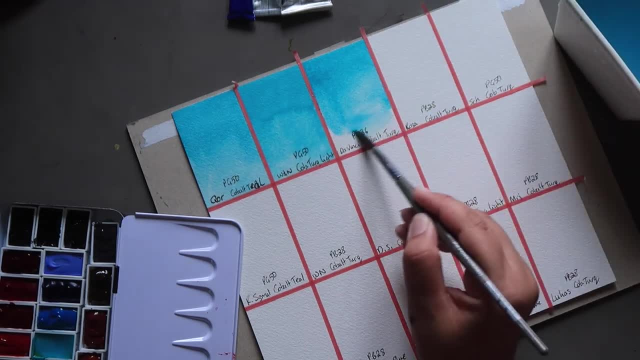 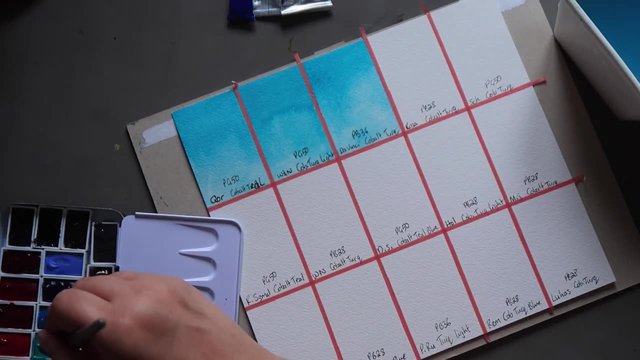 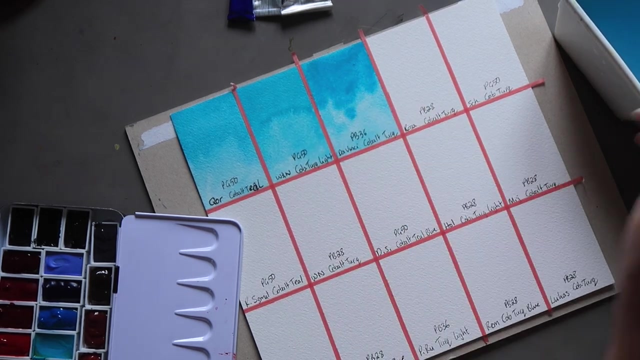 typically used to create a cerulean shade. as I said, usually cobalt, um sorry, cerulean blue chromium is the one that I've seen it in most, and again, this is a fairly green shade. next we have Rosa Gallery. there's down here. they call theirs cobalt turquoise. 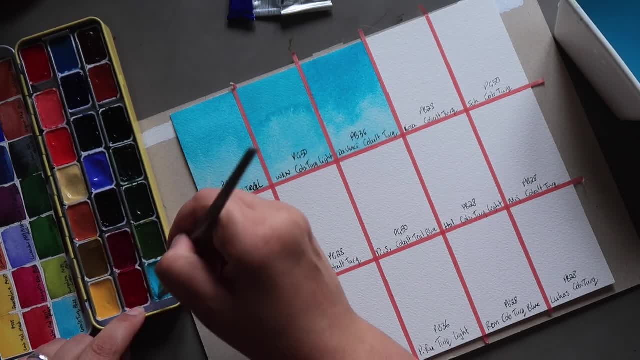 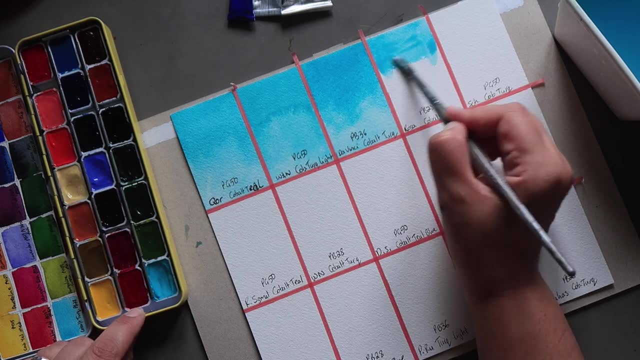 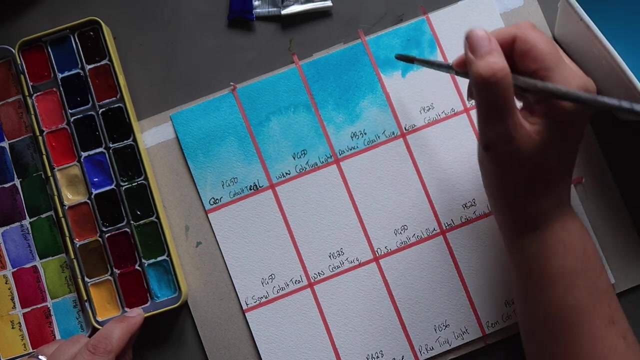 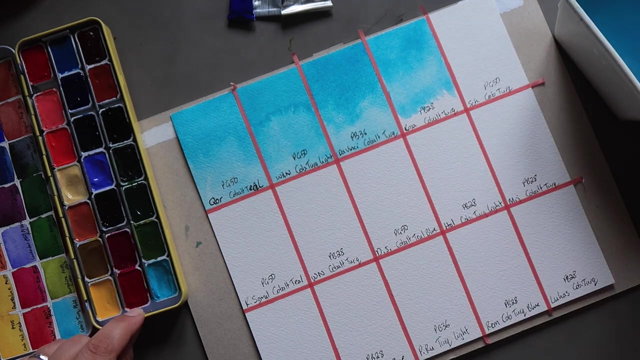 and their version is PB 28, and PB 28 is usually just used for straight up cobalt blue, but, like I said, some brands use this pigment also for their cobalt teal to cobalt turquoise color. it really just depends on how they're used and how the color's been processed, or the pigment, or rather, has been processed. 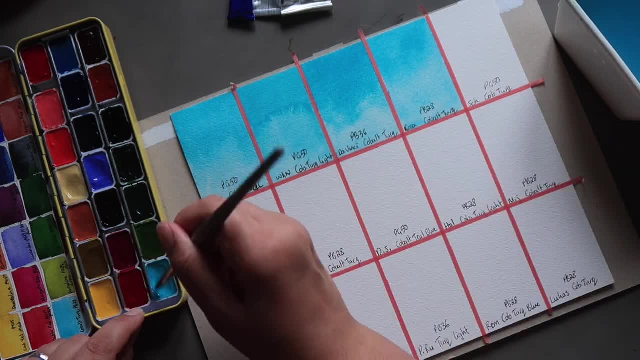 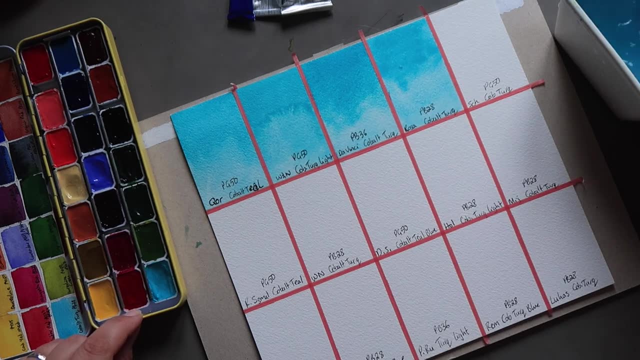 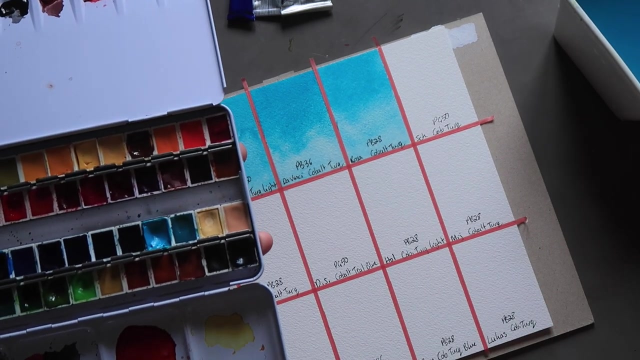 to determine what shade it comes out. as I say, this one's definitely on the lighter side in terms of pigment and color saturation. right off the bat it doesn't feel like it's super saturated. finally, for this row, we're going to be taking a look at schmincke's cobalt turquoise. their version is PG 50 as well. 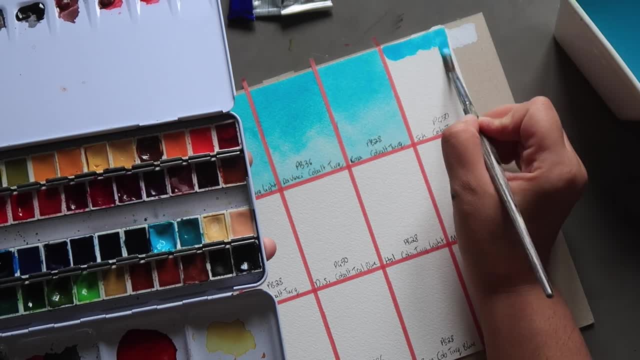 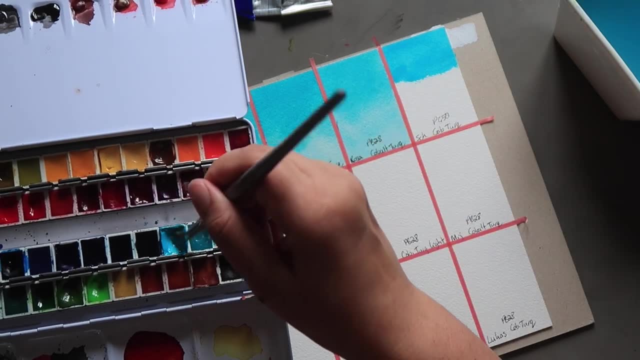 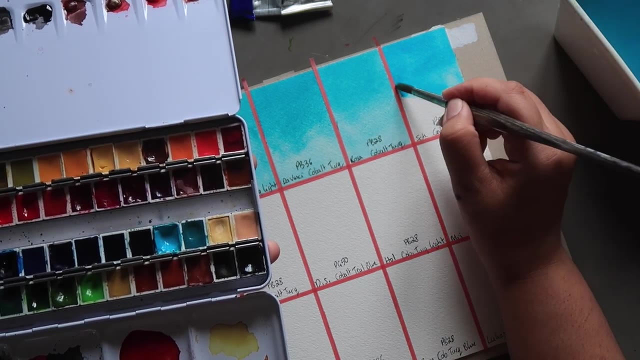 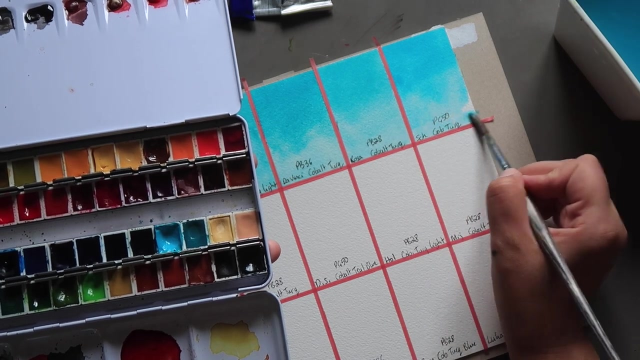 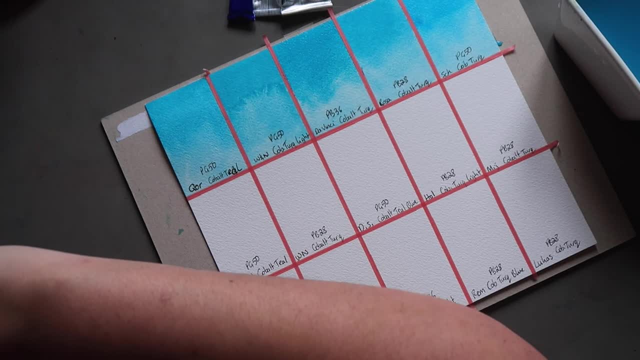 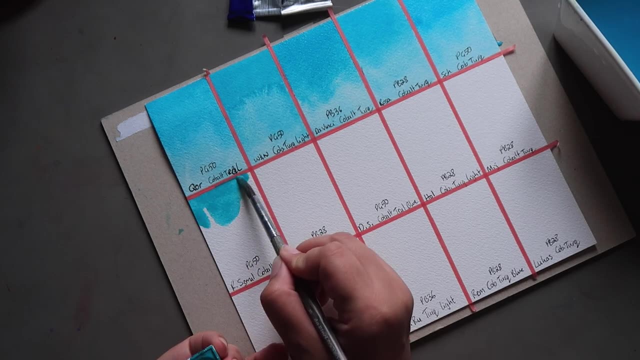 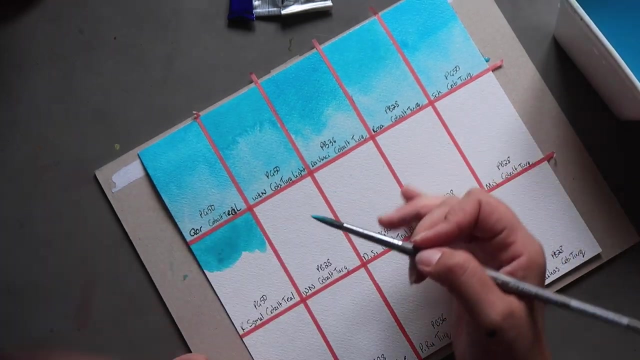 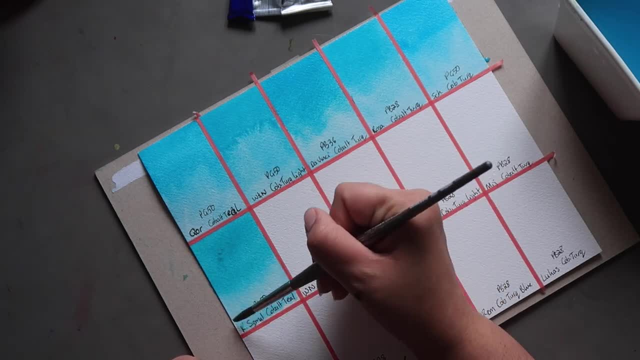 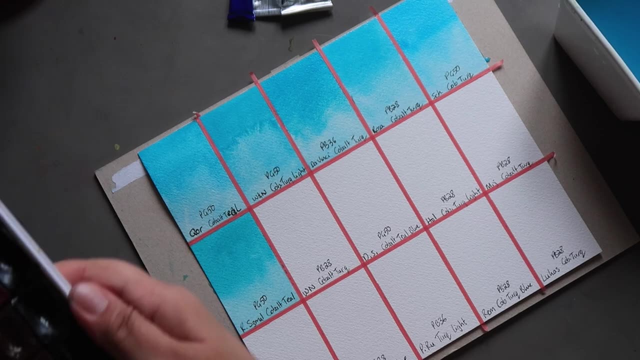 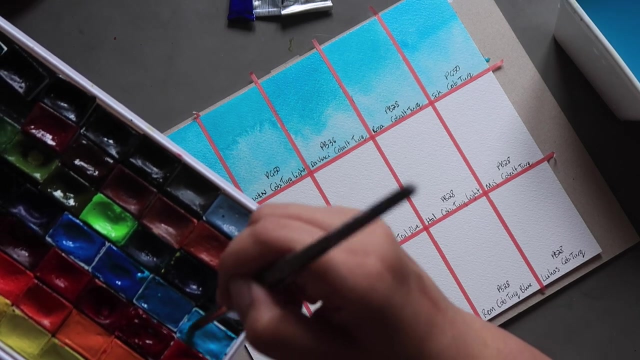 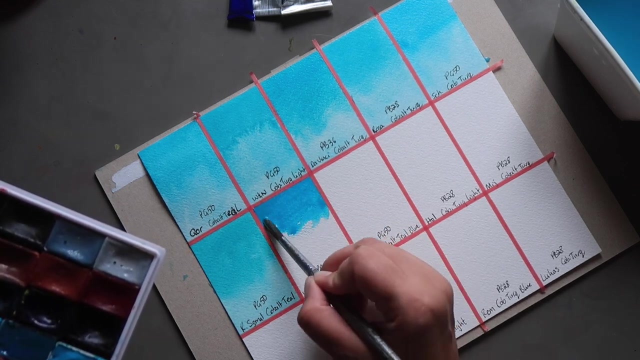 then we have the White Knights: Cobalt Turquoise, and that's just on the end here, and their version is PB 28, so this one's definitely fairly saturated and definitely more blue. so I'd say this one's a little bit more greenish than some of the others. I'd say 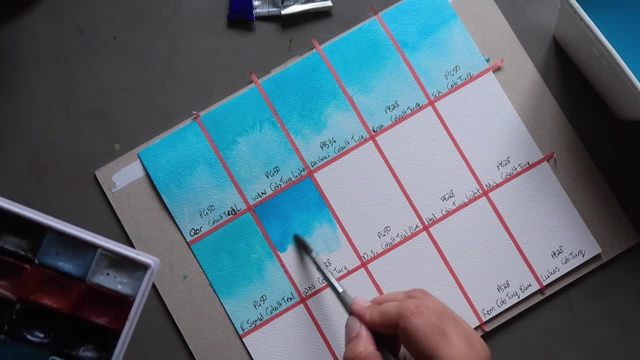 then we have the White Knights- Cobalt, Turquoise, and that's just on the end here. then all of the others we've looked at so far. I think you can see that on camera this looks a lot more blue than the others. have a bit more green. 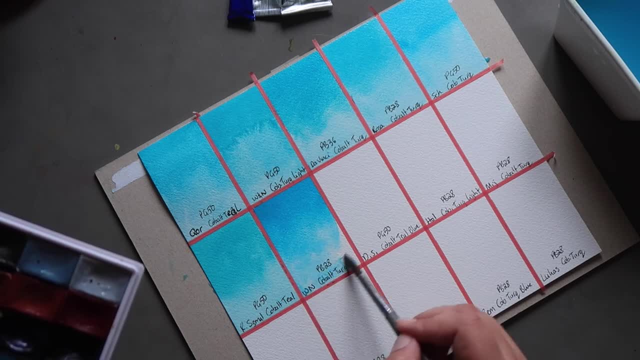 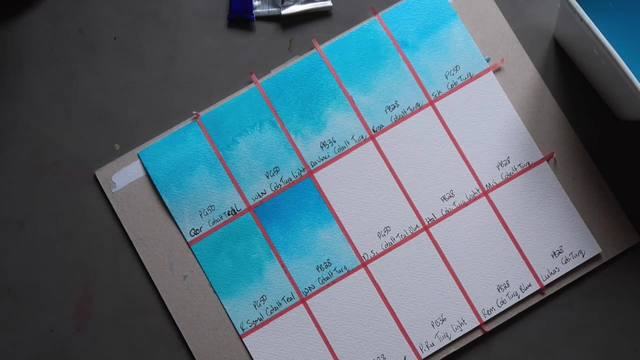 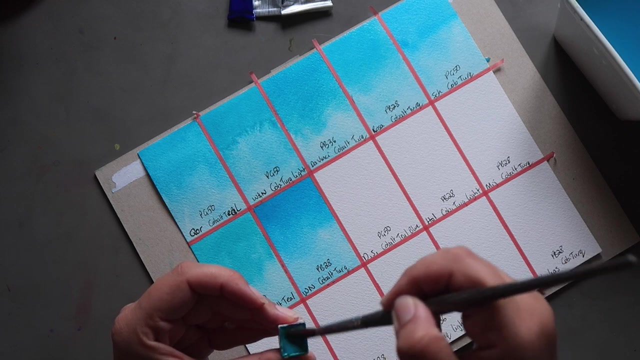 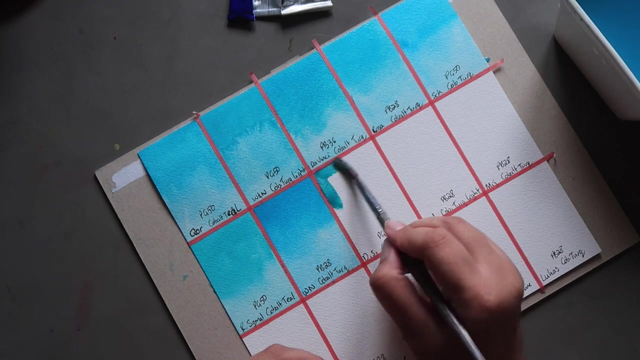 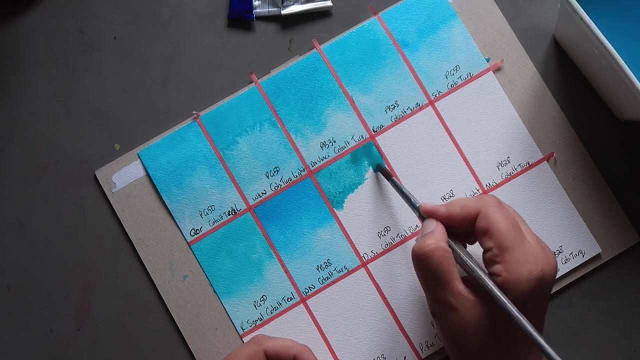 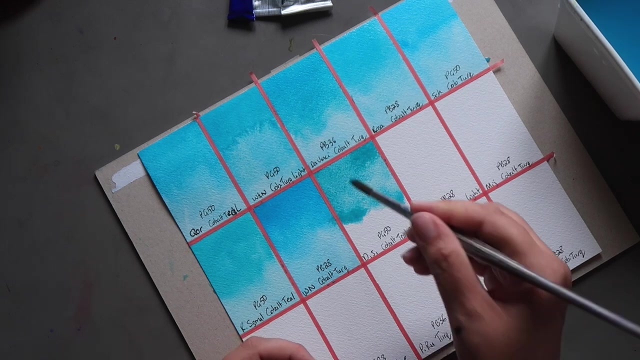 undertone to them. next up, we have the Daniel Smith Cobalt Teal Blue. I think, if I'm not mistaken, this is the one that comes out the greenest, and this one has a very strong granulation as well. yeah, this is definitely greener than all of the others so far. 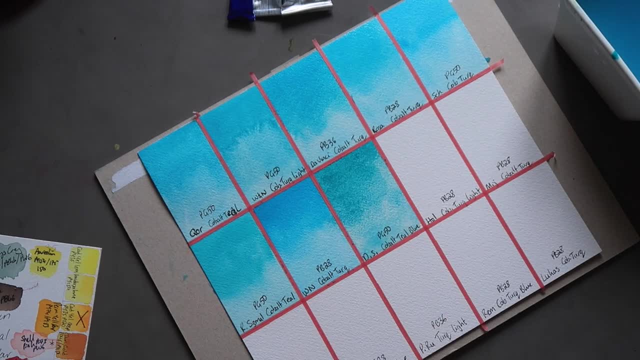 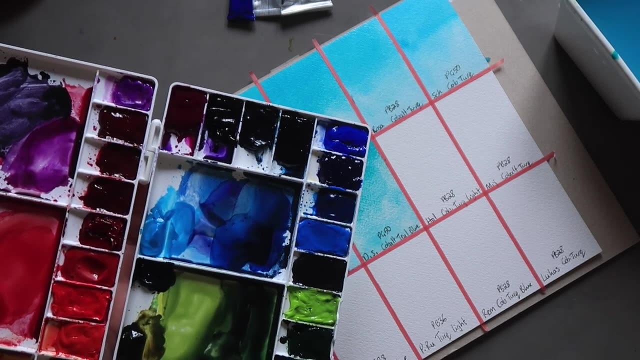 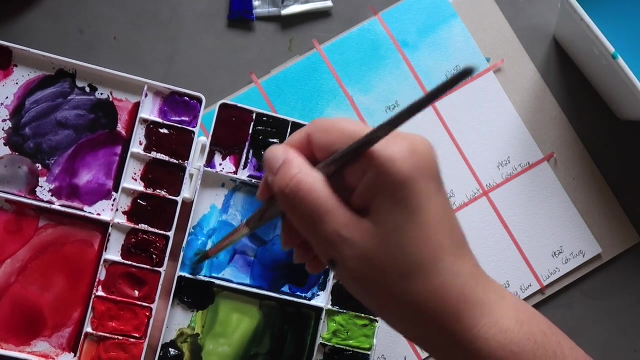 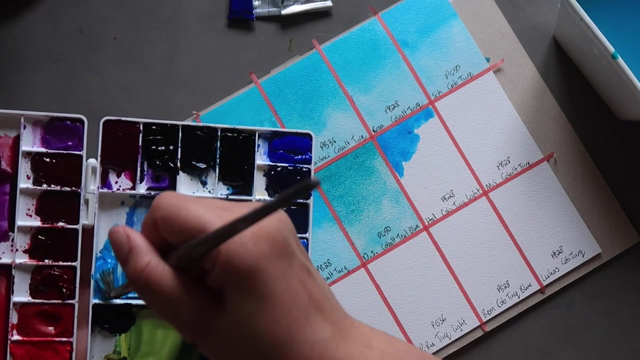 then we have Holbein. if I'm not mistaken, this one's also fairly blue. yeah, this is definitely greener than all of the others so far. Holbein's version of Cobalt Turquoise Light is PB 28. I don't know if I mentioned the Daniel Smith one is PG 50. I didn't mention it. 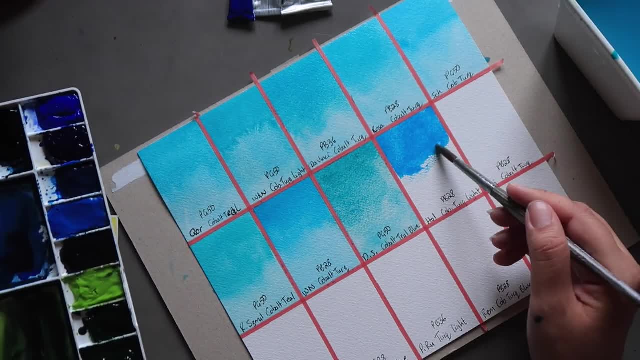 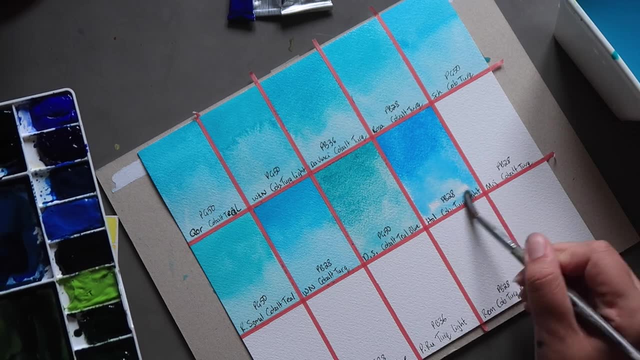 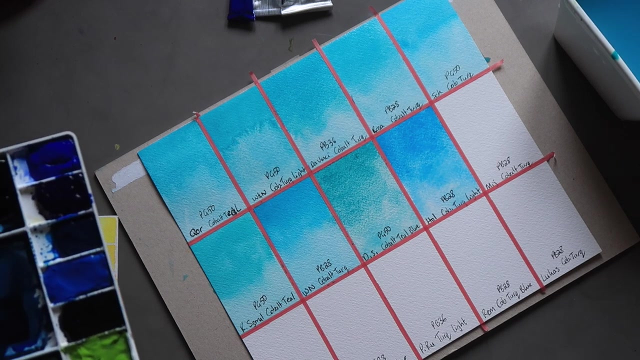 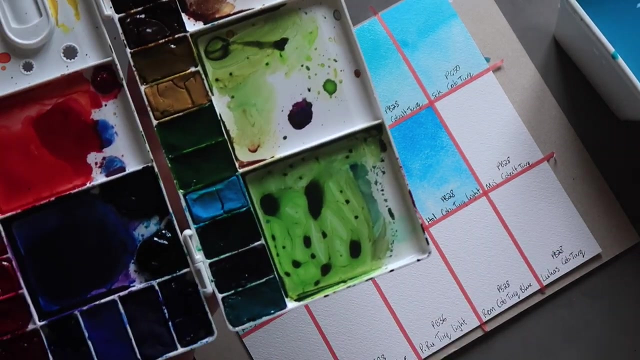 yeah, this one's very blue again, compared to a lot of the others, especially compared to the Daniel Smith one next to it to it, That Daniel Smith one is already granulating quite a lot. Next up, we have Mugello's Cobalt Turquoise they call theirs, and this is also a PB 28 pigment. 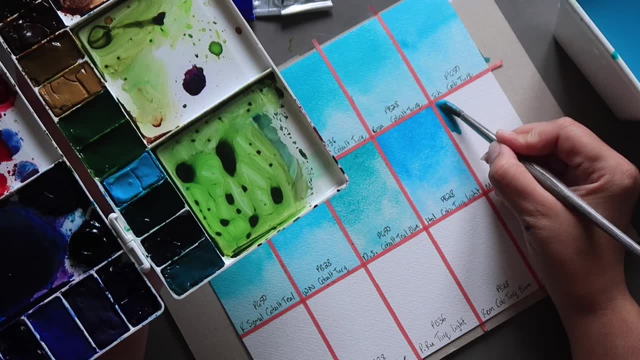 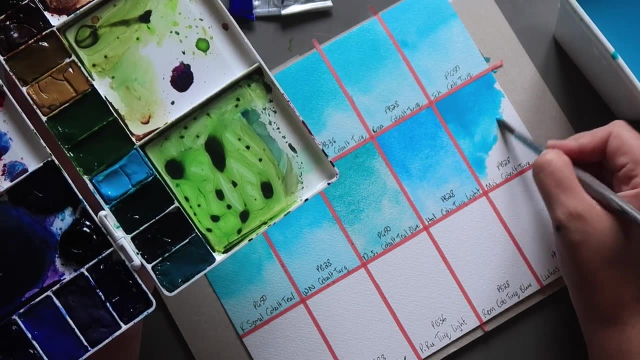 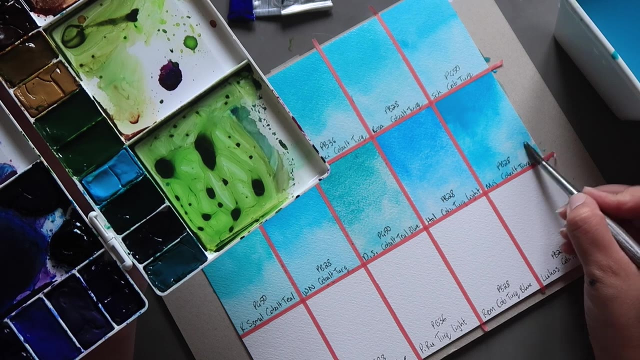 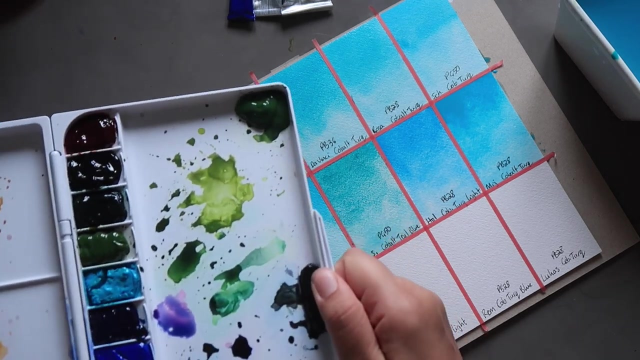 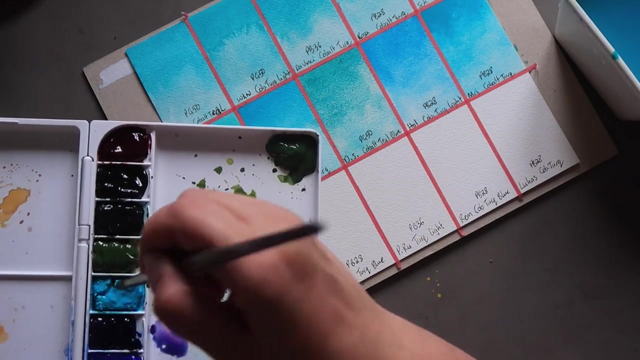 This one's a bit more green than the Holbein, not quite as blue, but not quite as green as the Daniel Smith. Then we have Sennelier. their version is called Turquoise Green. Okay, While Sennelier colours usually stay quite tacky, this one does dry quite hard. It re-wets. 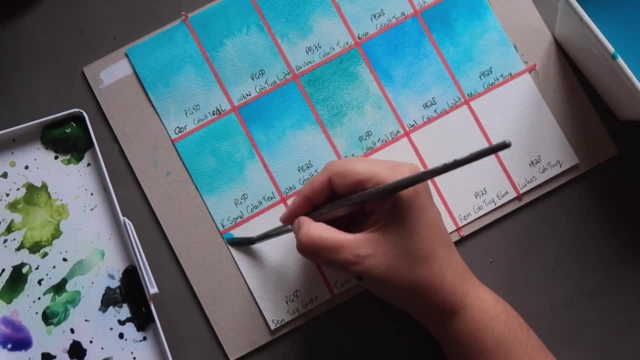 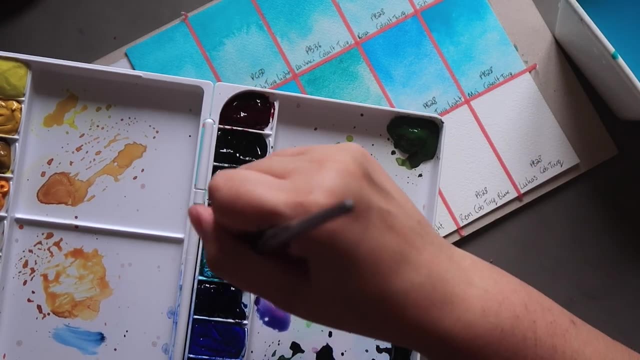 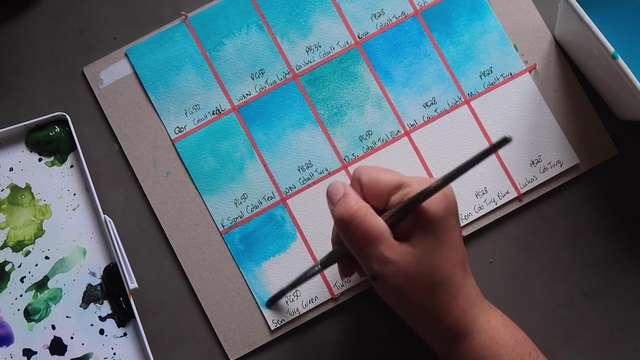 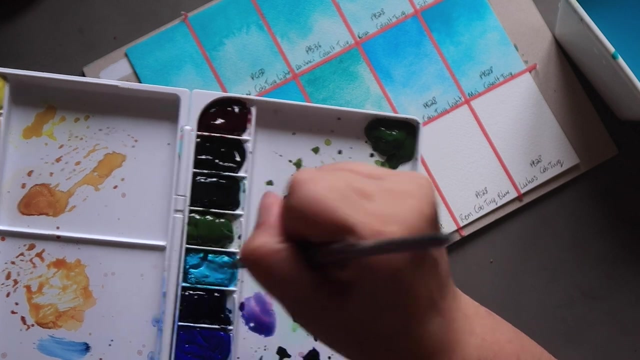 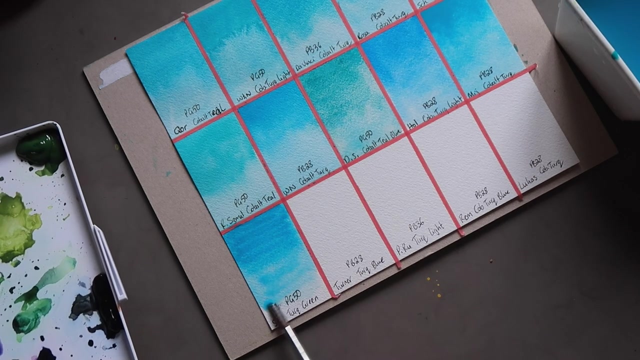 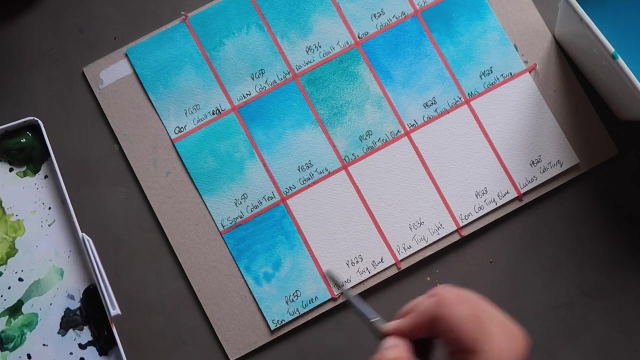 beautifully, but it does dry quite hard. There's his PG 50,. it's definitely on the bluer side, Okay, And their one does granulate as well. All of them granulate to a degree, some just more so than others. 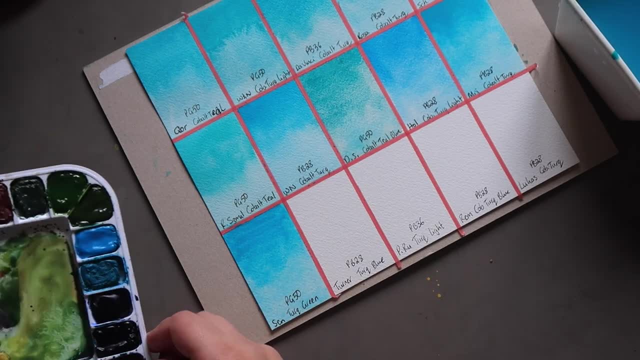 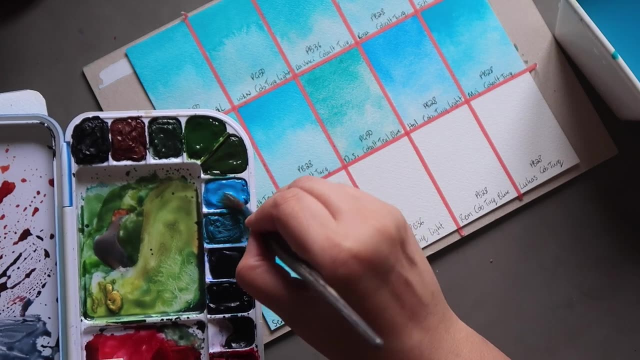 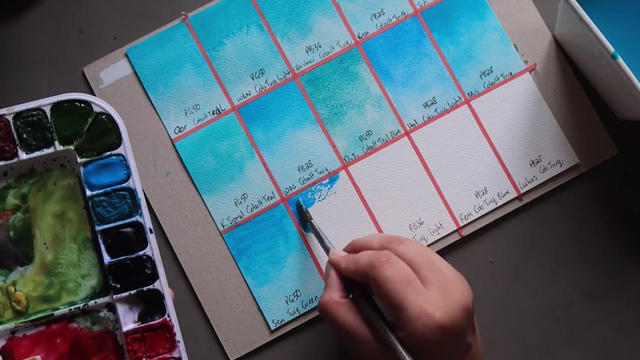 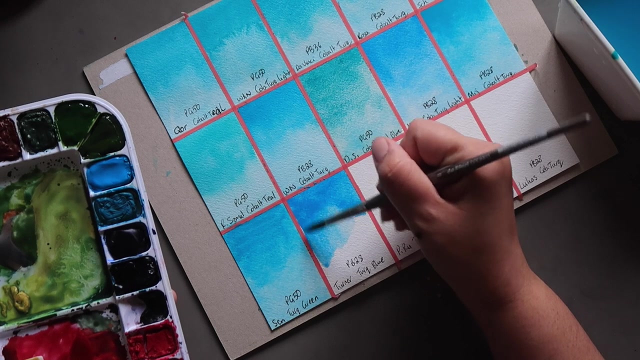 Then we have Turner's version. they just call theirs Turquoise Blue. It's also PB 28, and this is definitely one of the cheaper variations of the Turquoise Blue. Okay, It's quite a blue one as well. it's very blue leaning. it's not as green as some of. 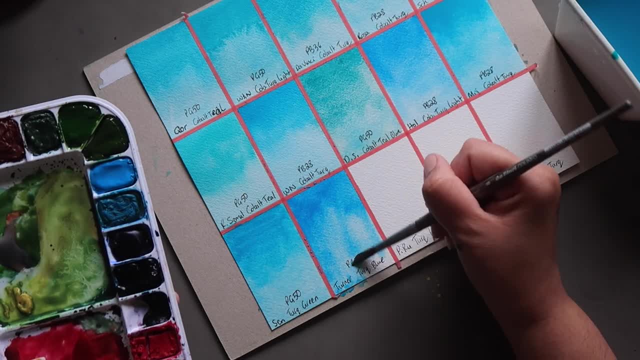 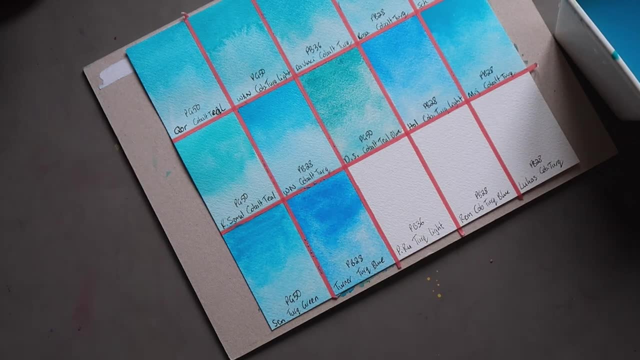 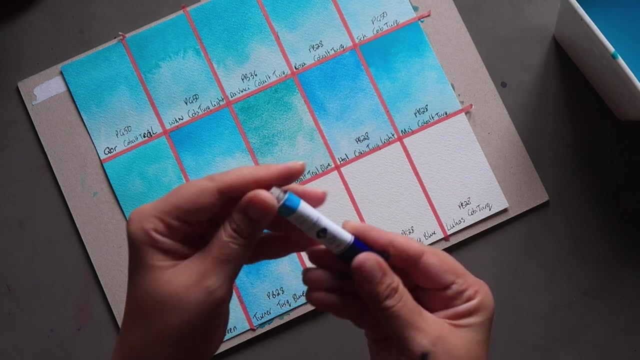 the others. so, depending on your colour preferences and how, where you like it to land on that scale of blue to green. Okay, I have in tubes. they don't currently live in palettes at the moment. so we have Paul Rubens and theirs is called Turquoise Light and it is the pigment PB 36.. 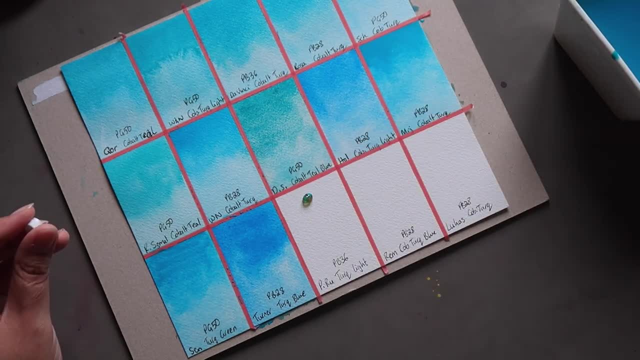 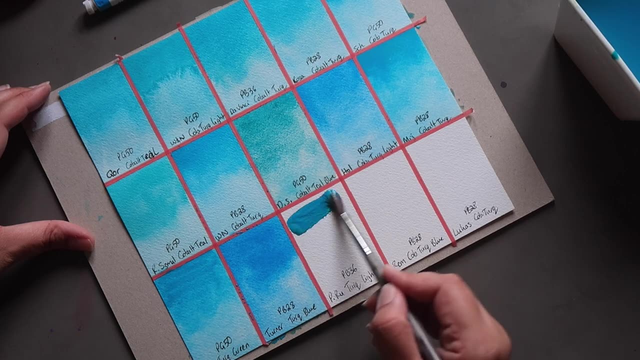 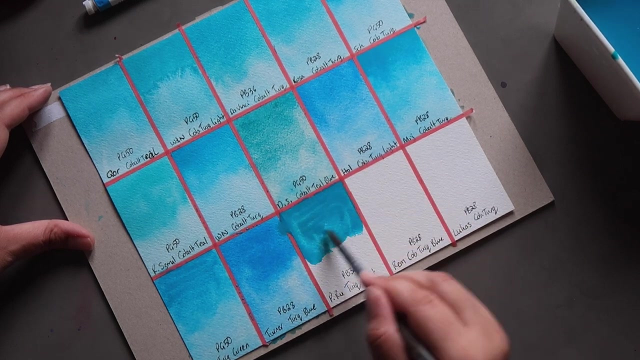 Oh jeez, a bunch of Gamera coming out first. Okay, Hopefully that doesn't affect the colour too badly. A bit too much pigment there. Okay, Sorry, a little bit went over onto that Turquoise Turner version. Okay. 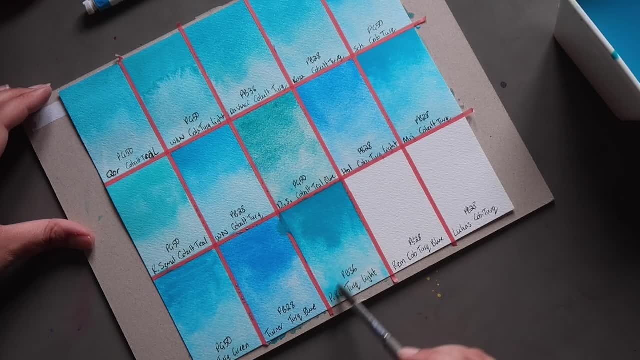 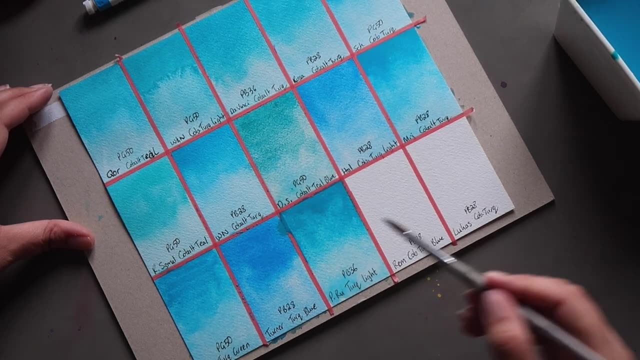 And again. so this is a nice greener version, greener leaning, Trying to get rid of some of that excess pigment. So the only problem with doing it straight out of the tube is they are going to be a little bit more stronger. 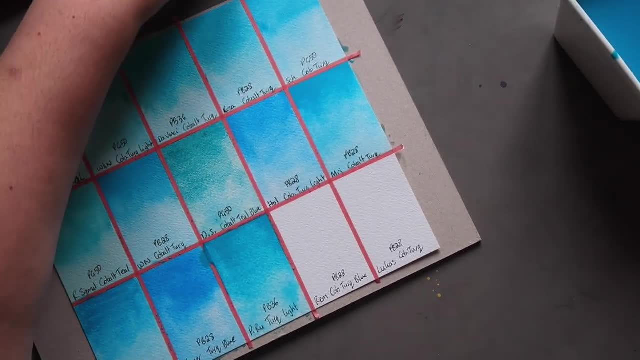 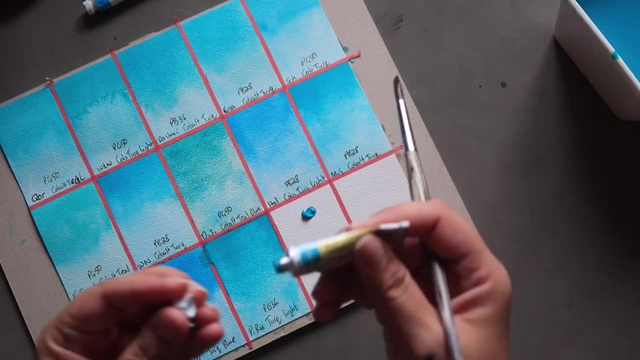 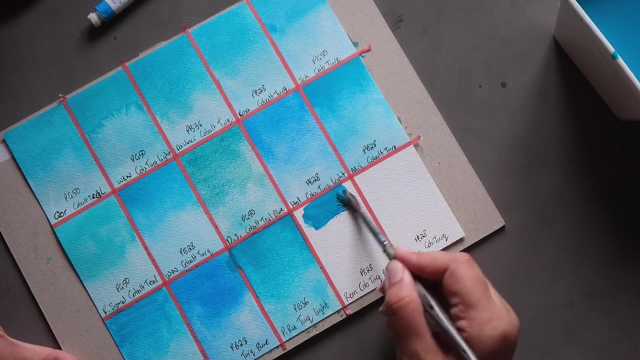 Okay, there we go. Then we have Rembrandt Theirs is called Cobalt Turquoise Blue Theirs is also PB 28. So I think this is a slightly bluer version. Okay, Okay, Okay, Okay Okay. 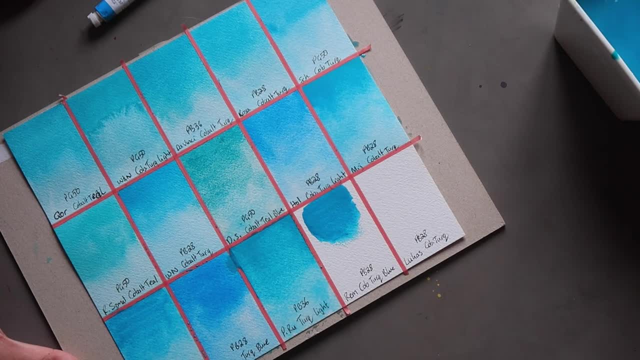 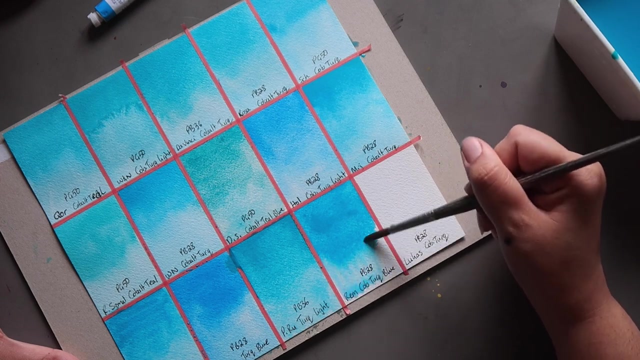 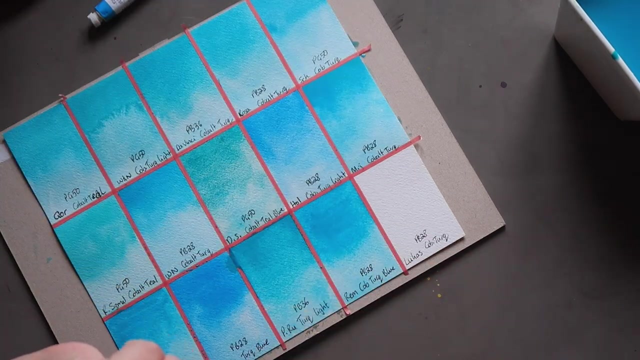 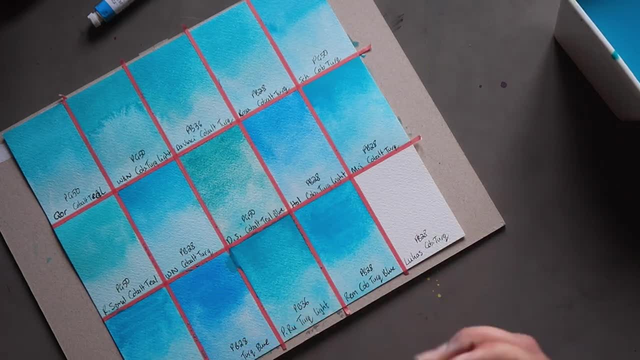 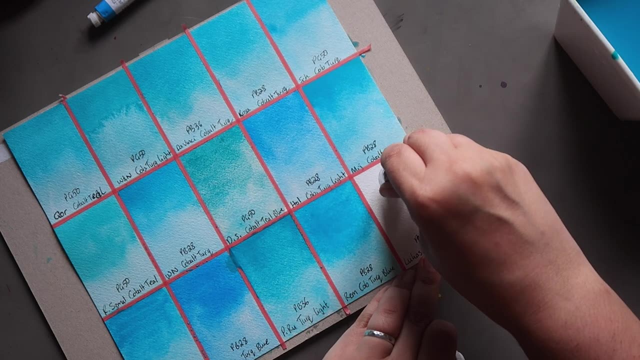 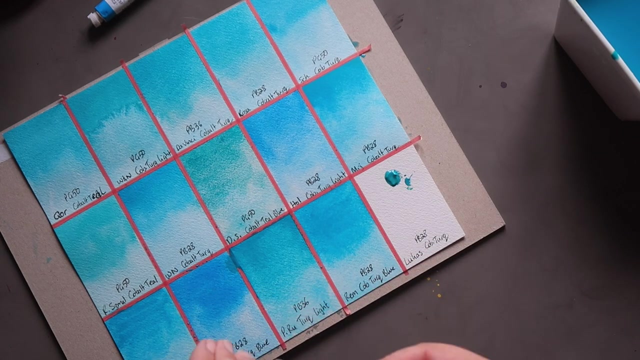 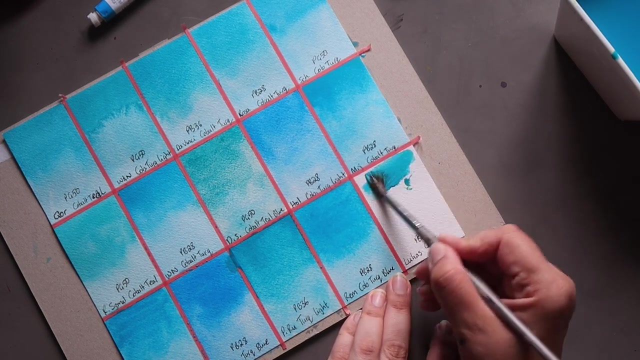 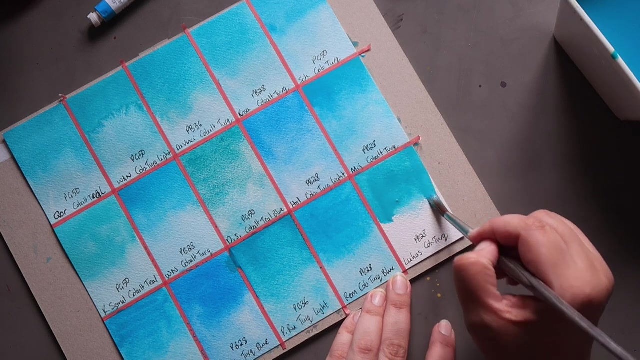 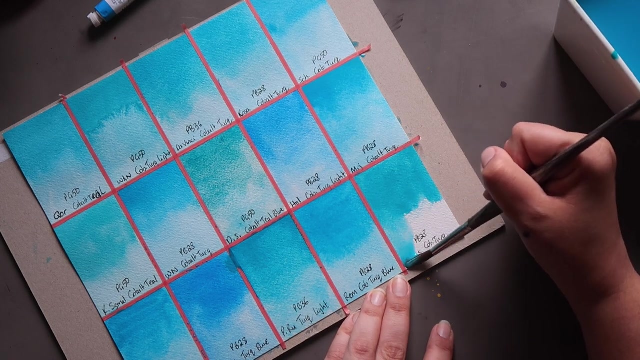 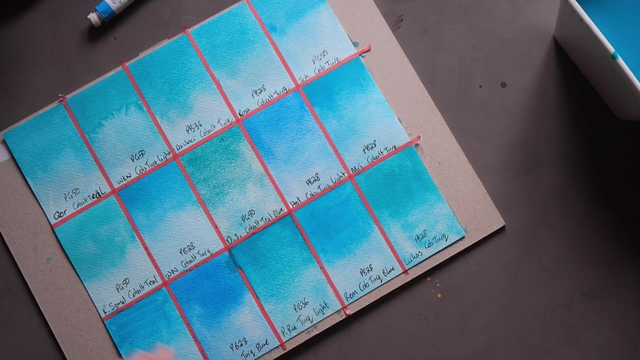 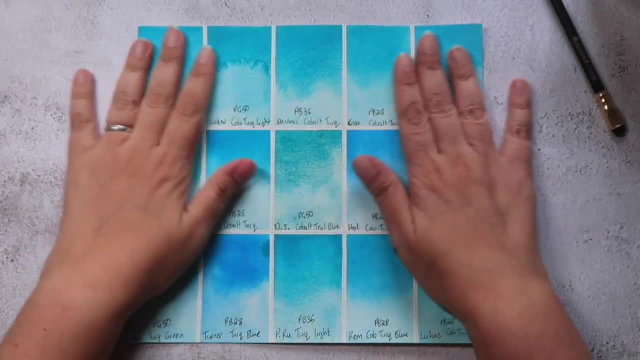 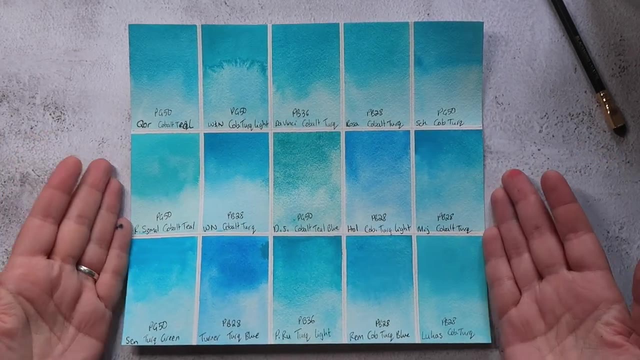 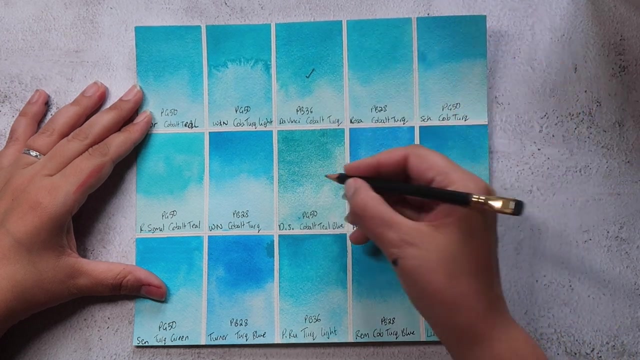 okay. so our swatches are all dried now and you can see there is quite a range in hues of this sort of cobalt turquoise, cobalt teal shade color that we're looking at here today. right off the bat, i will tell you my favorites are the da vinci, daniel smith, even though this is. 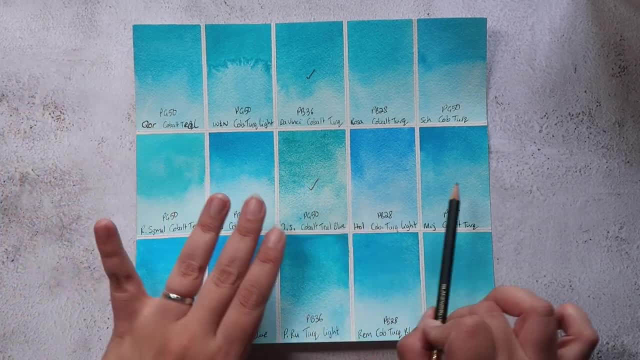 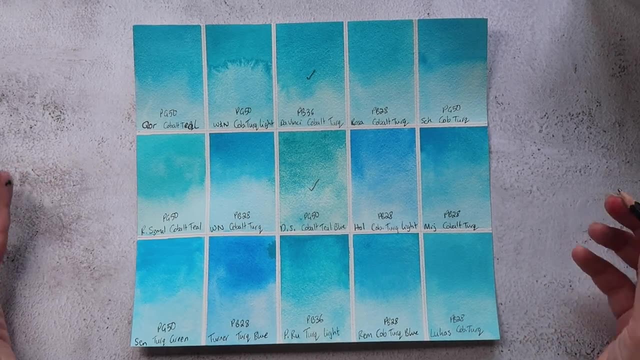 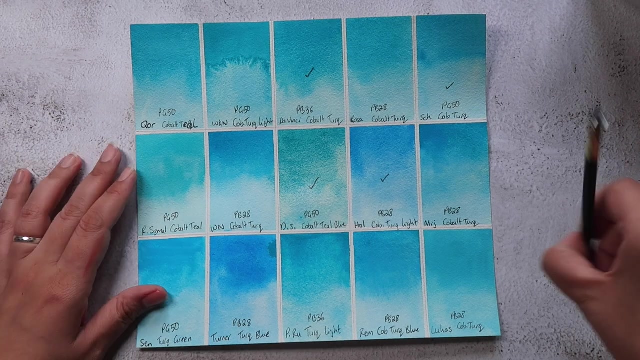 the greenest of all of them and i definitely prefer that somewhere in the middle. the granulation in this one is absolutely insane. um of the bluer ones, i really like the holbein and the schmincke. one has a really nice delicate touch to it. um, i do like the roman schmalt cobalt teal as well. 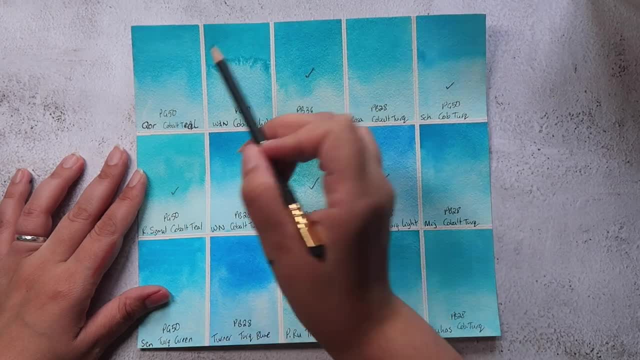 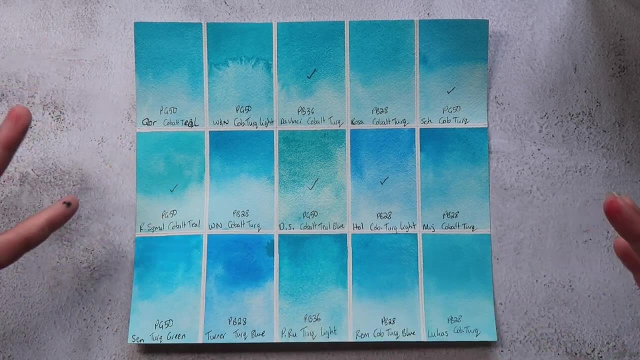 the core is beautiful, but, like i've said in previous videos, i just cannot justify the cost of purchasing a tube of core paint here in the uk, unless you're buying it as part of a set, which is how i got this one, or it's been gifted, or if i'm traveling to the us, it's not one i would pick up locally. 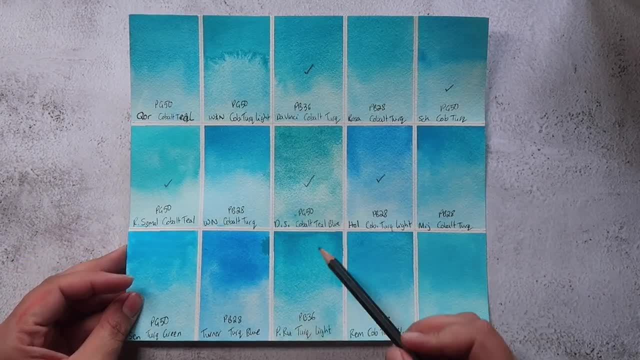 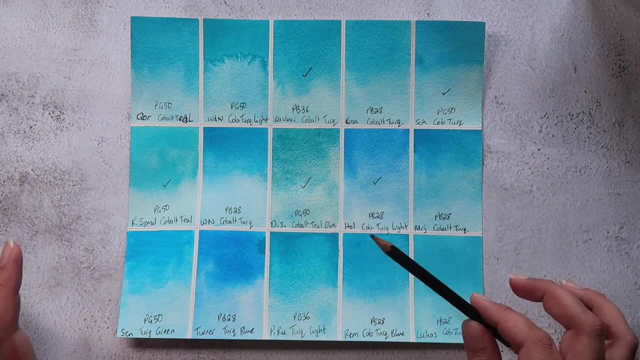 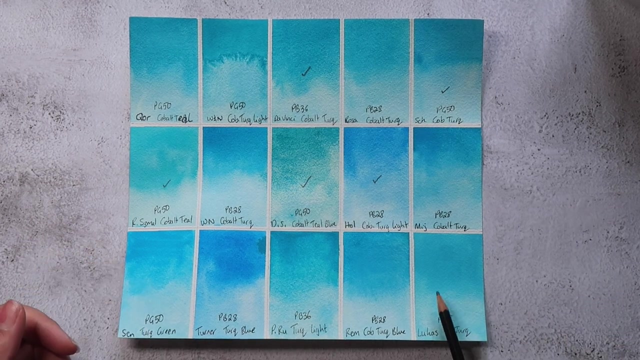 um, even the paul rubens turquoise light is fairly granulating, although it's slightly milky in the um when it dries down. same i would say with the sommelier, although for some reason that one doesn't bother me as much, and the lucas is very milky once it's dried down. i'm going to try and show you so you can see. 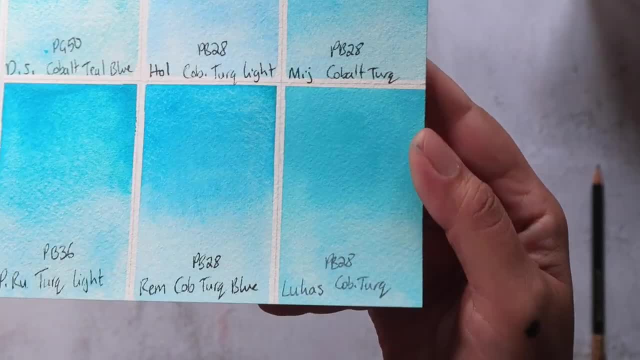 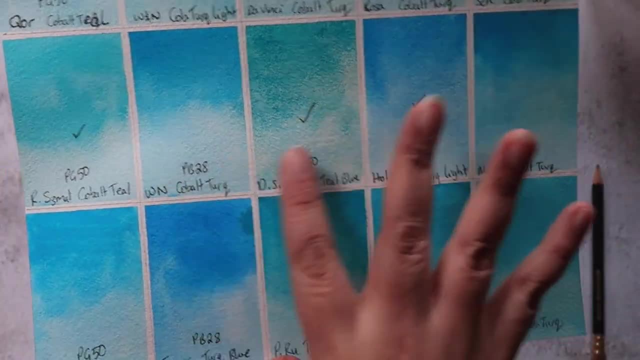 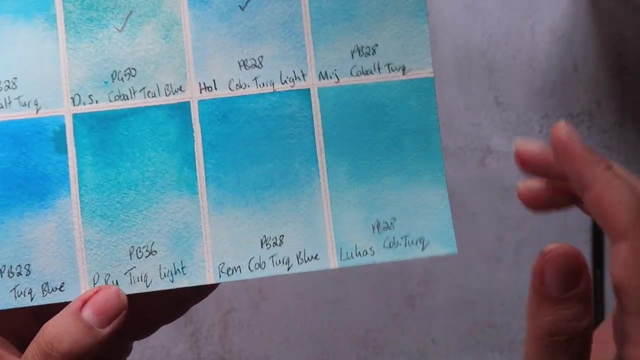 what i mean. it's just dried very milky like it's got sort of a milky cast to it compared to some of the other ones. even though this is a semi-opaque color you can see in a lot of the other swatches the writing is still very clear, whereas here the black line is a lot more obscured. so i don't know. 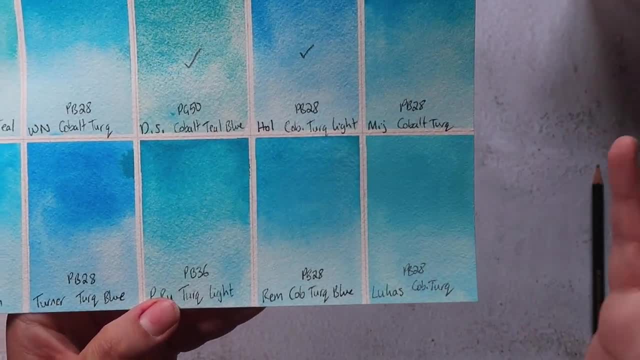 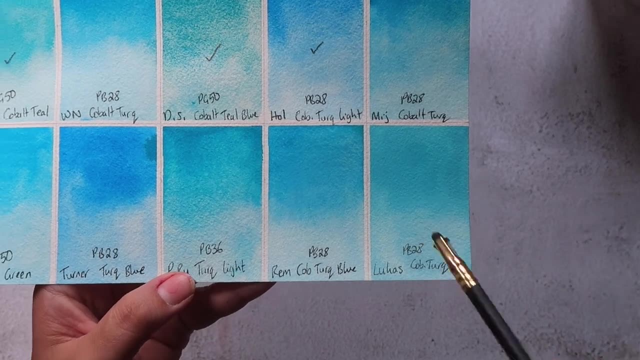 i just don't like it. i i used to think this was a really lovely color and i i do love this. i'm going to show you what i did love this and i thought it was really good value for money, which it is, but seeing here now, compared to all the others, it's a no for me. uh, the turner, which is also. 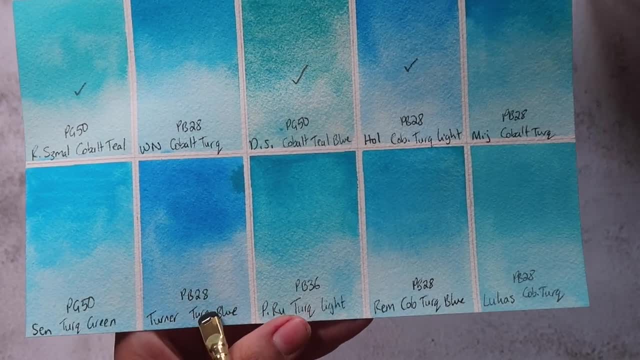 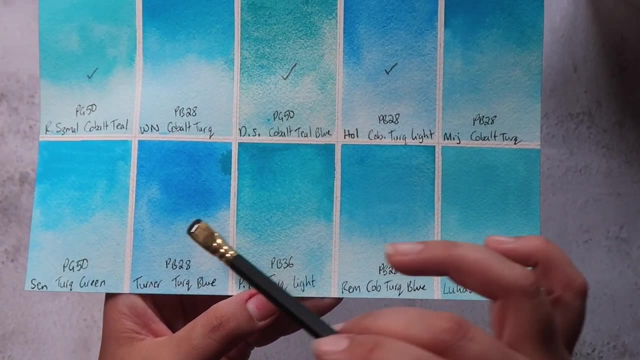 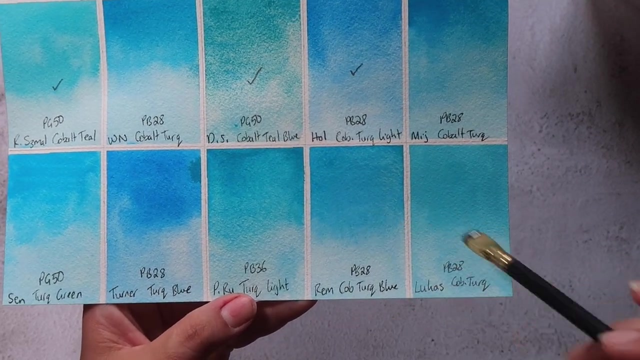 really affordable. it's a bit bluer but it's a lot cleaner looking and i would say, if you're looking for an inexpensive cobalt turquoise, teal color, i would say this one is better than this one. the turn is better than the lucas, in my opinion. um, looking at the for 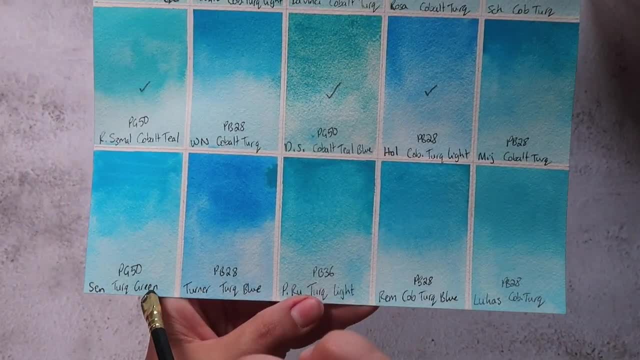 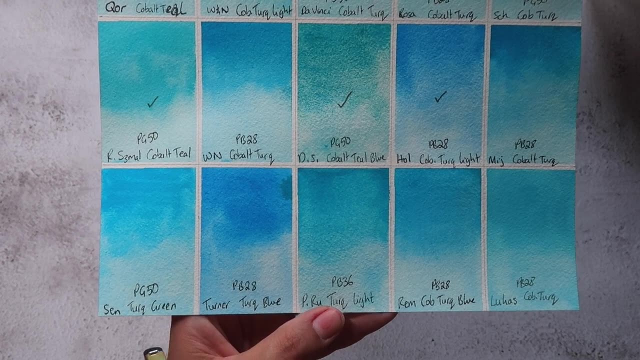 all of the, although sennelier is also quite affordable here in the uk and in europe in general, and i do like this one. it's got a little bit of cloudiness to it in the mass tone, but it has a really nice granulation and mixes really beautifully, and this is also one that i really